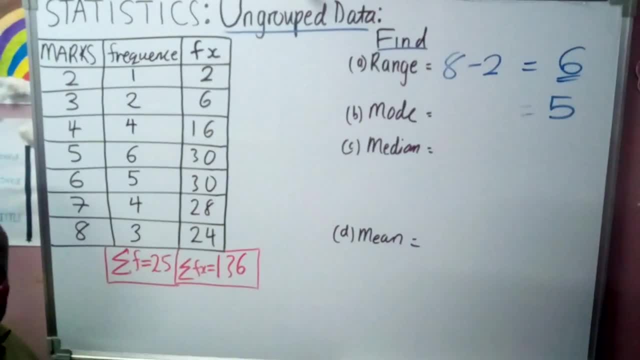 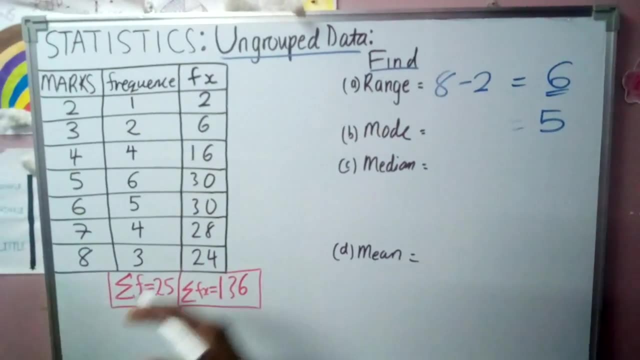 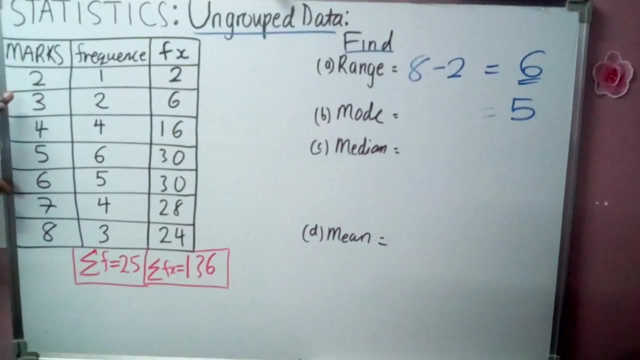 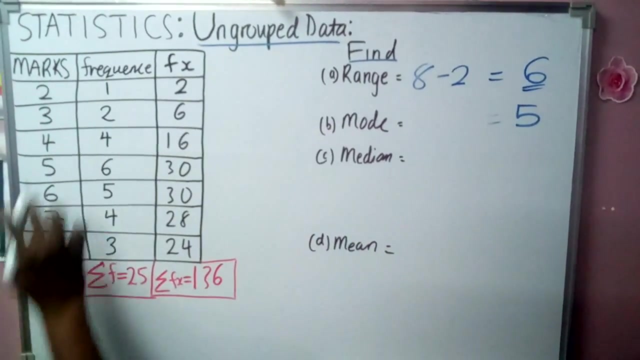 Now median. Median is the data which is in the middle, After arranging all the data in order. Now, when you look at our data, we have 2 repeating 1 time, 3 repeating 2 times, and so on. 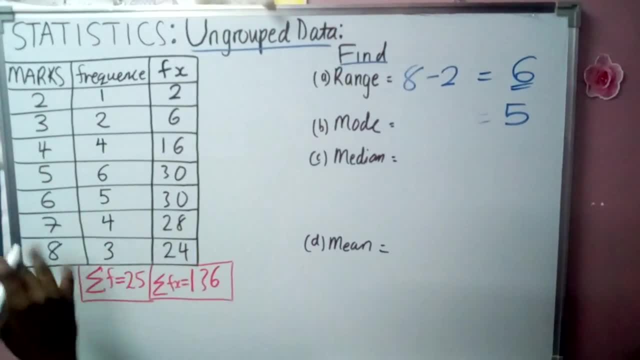 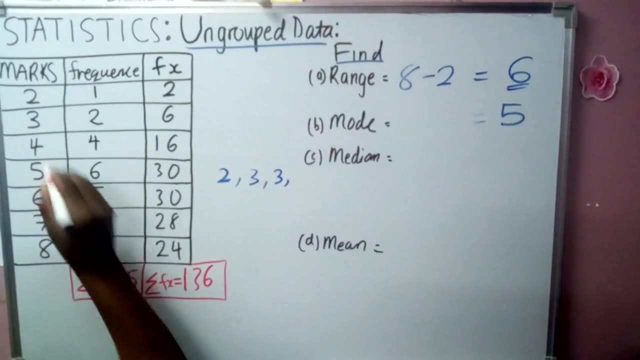 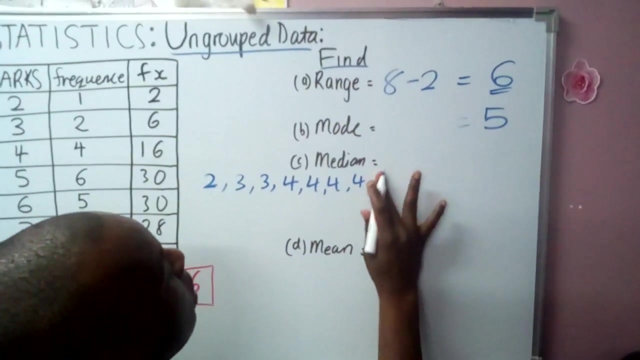 We can have 2 methods. 1 method: we can list all this data: 2.. 4 is repeating 1 time. 3 is repeating 2 times. 4 is repeating 4 times. 5 is repeating 6 times. 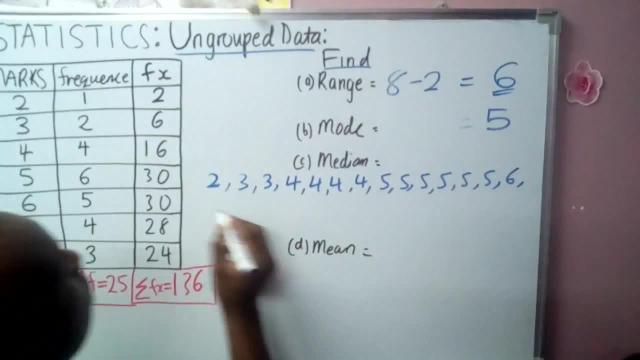 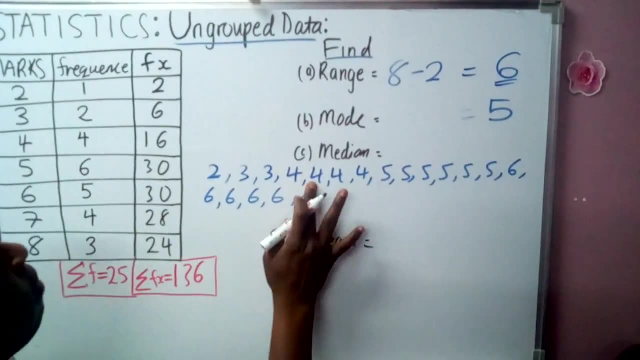 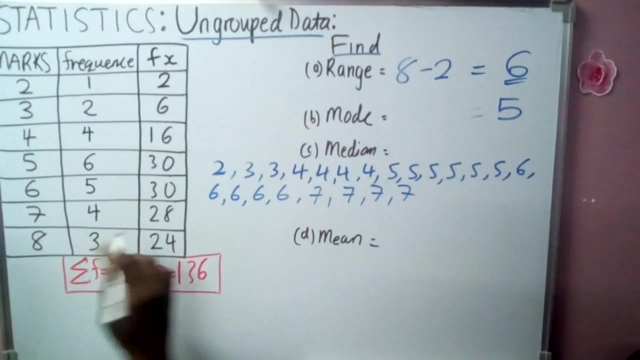 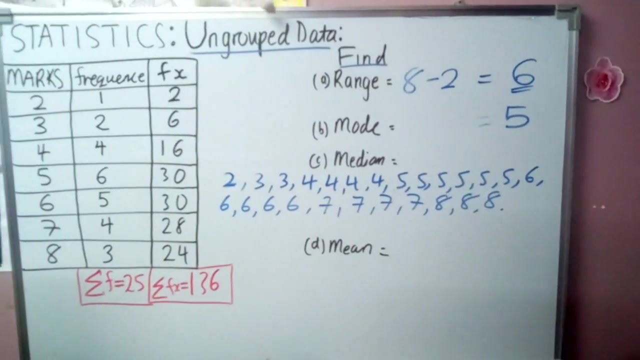 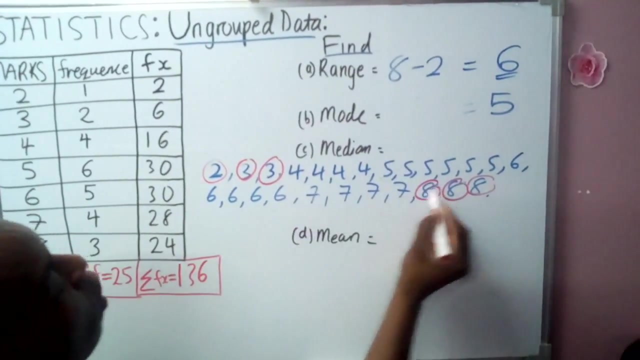 6 is repeating 5 times: 1,, 2,, 3,, 4, 5.. 7 is repeating 5 times, 8 is repeating 4 times And 8 is repeating 3 times. Now, after having all our data listed, then we start cancelling one by one until we get the middle data. 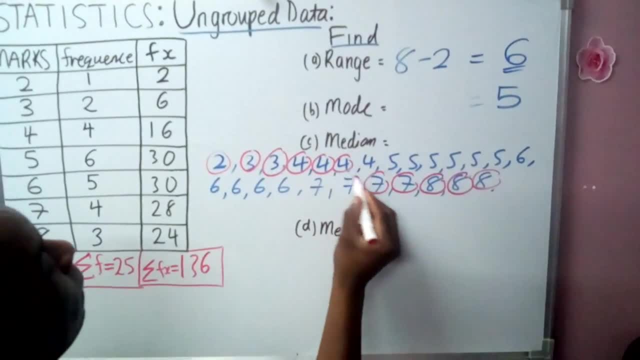 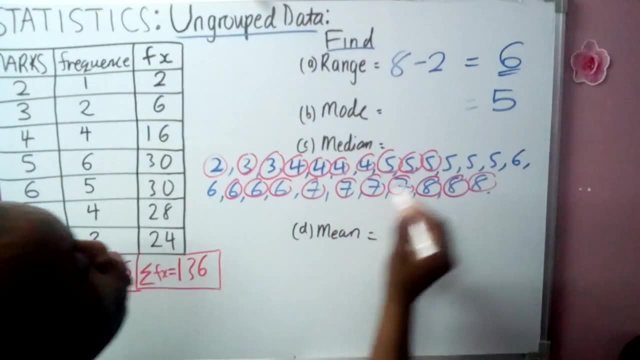 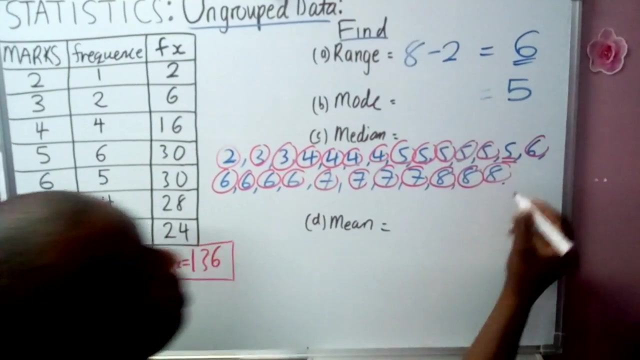 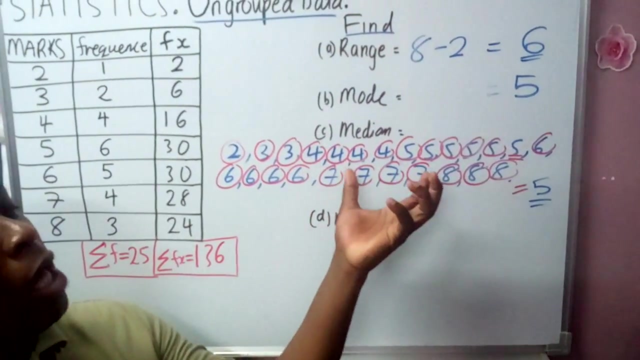 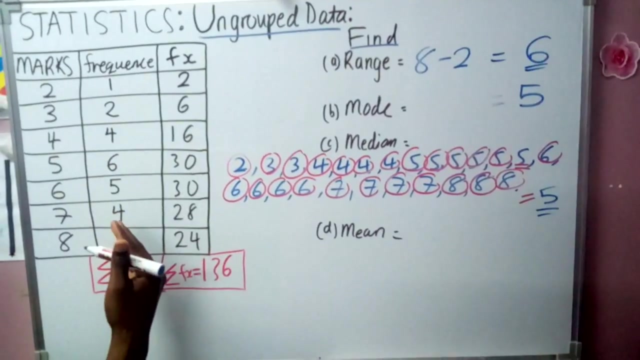 And finally, our middle data. The middle data will automatically be our median, And hence our median here will be 5.. However, we can find the median using another shortcut method: You take the sum of all the frequencies And remember: our sum of the frequencies is 25.. 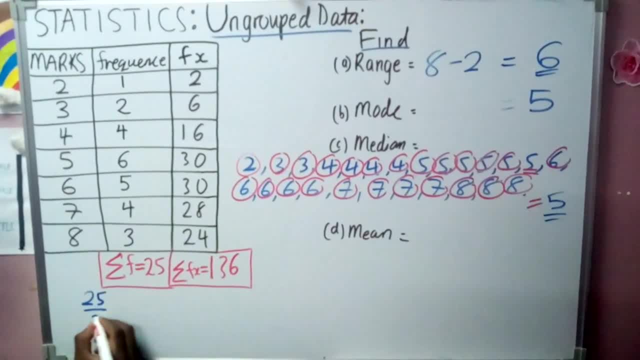 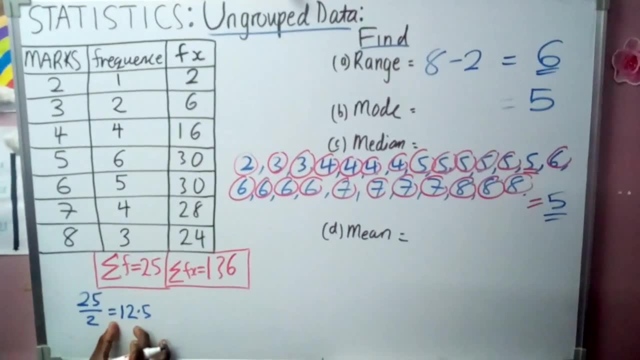 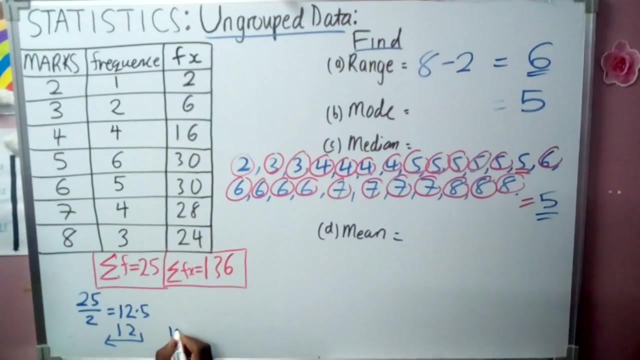 So we take 25.. We divide by 2. This gives us 12.5.. Now 12 is our full number. It means there are full data this side, that is, 12. And another full data that side. 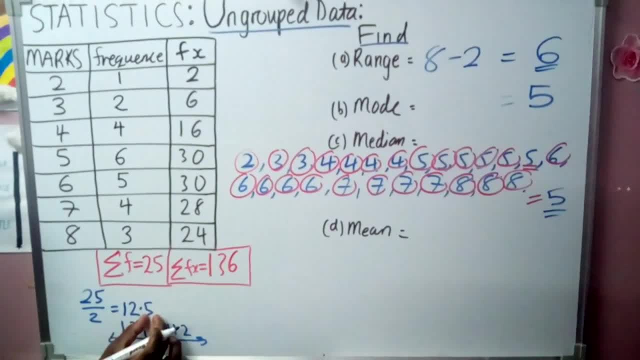 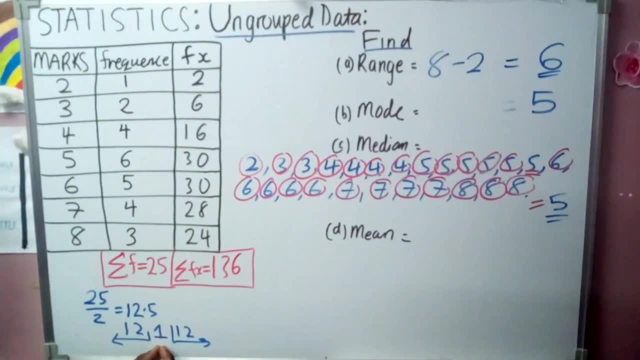 This gives a total of 24.. Now this 0.5. And another 0.5 splitted gives us the one data that is in the middle. Now, if the first data is total of 12. Meaning the next data will be the median.